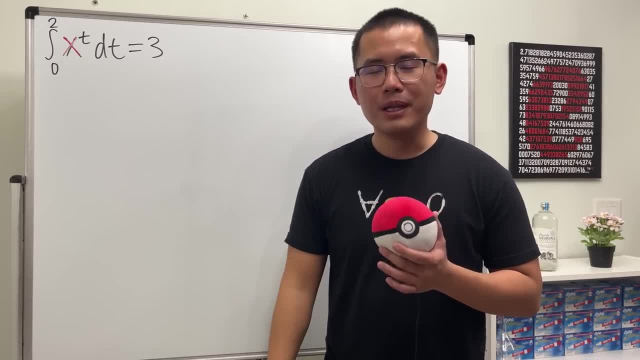 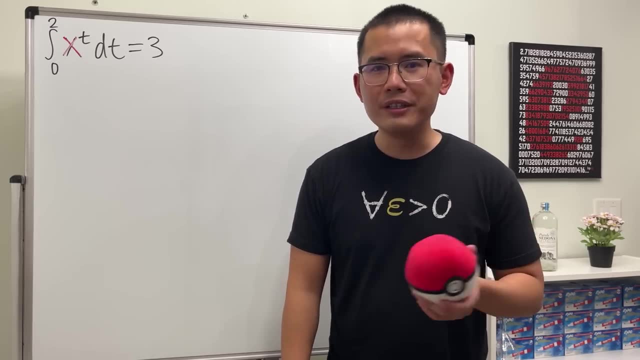 tell you this is going to be a very, very hard equation, because not only we have to use calculus, but also the Lambert W function with some technical part And, of course, most importantly, I came up with this And I'm pretty sure 99% of the world population wouldn't know this. 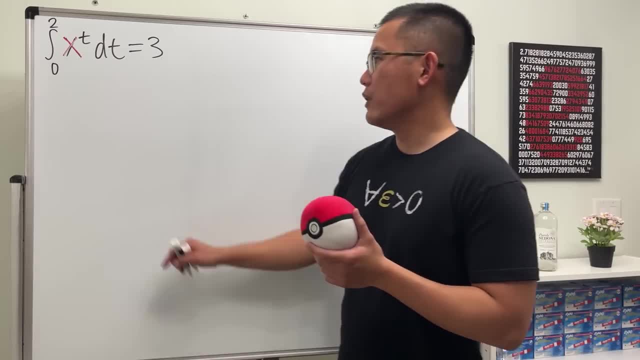 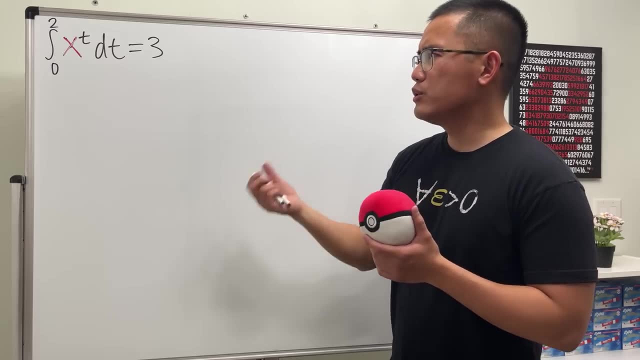 But anyway, let's see how we can deal with this. First off, we will have to know that this integral is in the t world and the x is just like a constant. So we can actually just integrate this, no problem with that. And let me just remind you, guys on the side, 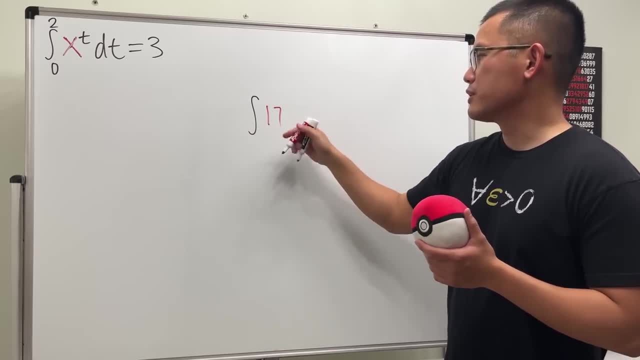 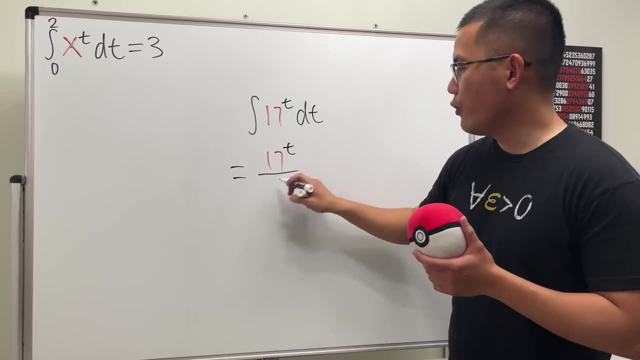 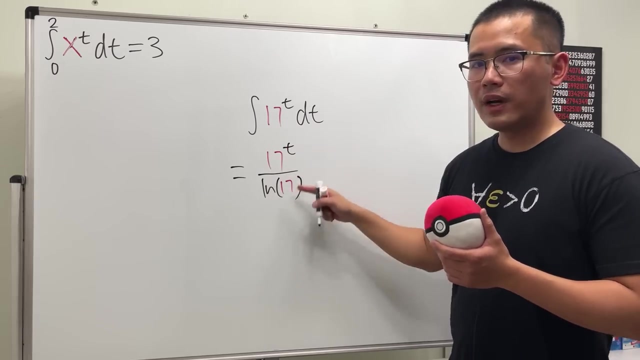 when we integrate, let's say 17,, which is just a constant raised to t's power, dt. This right here will give us 17 to the t's power over ln of the base 17.. So the exponential function: when you integrate that you keep it but you divide it by ln of the base. So in this, 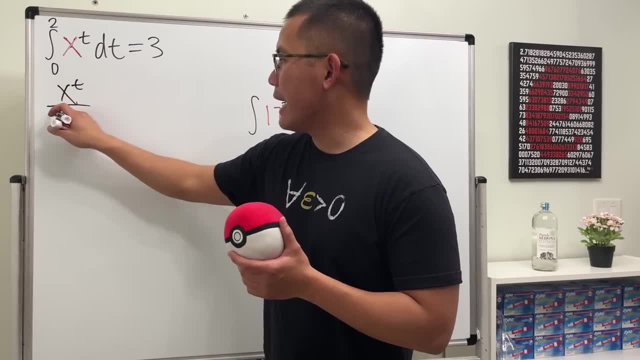 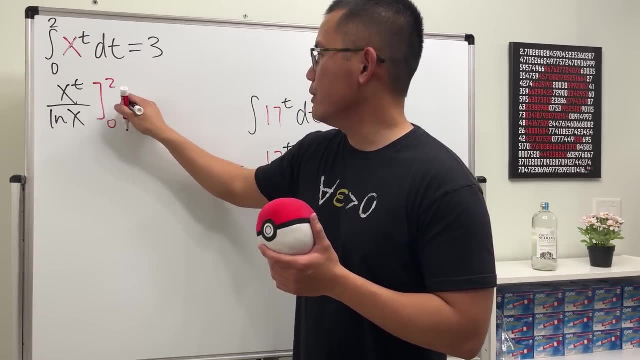 case, we will just have x to the t's power divided by ln x, And that's the calculus part. And then, of course, we'll just have to plug in, plug in 0 to 2, and then make this equal to 3.. 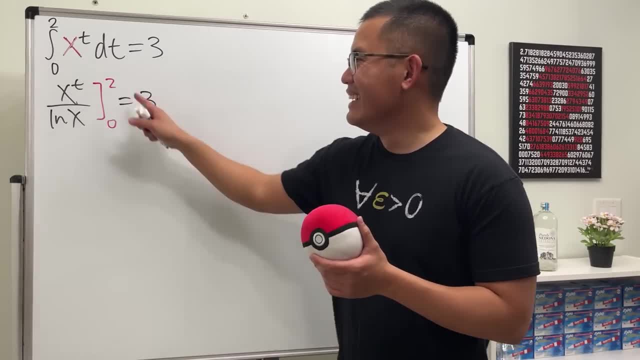 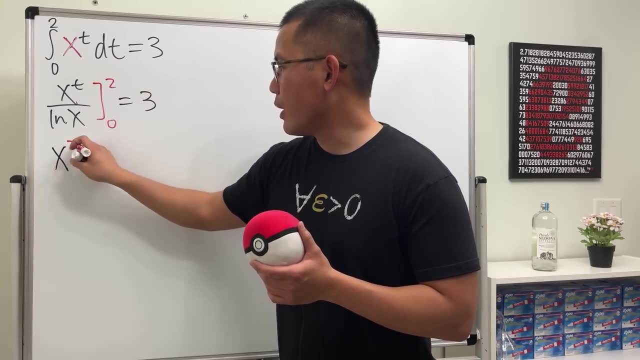 So that's what we have now. That's the calculus part. Remember we are in the t world, so we will have to plug in the 2 into the t. So first we get x to the second power and then minus, plugging 0 in here and x to the 0's. 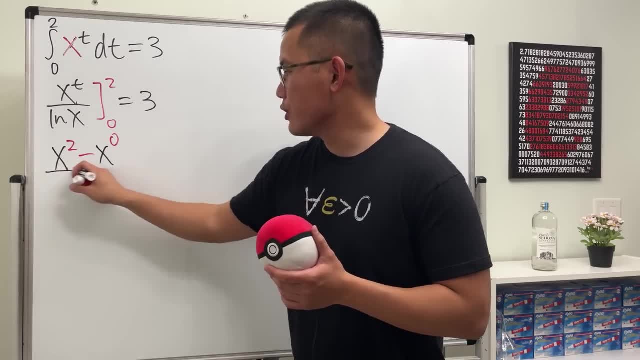 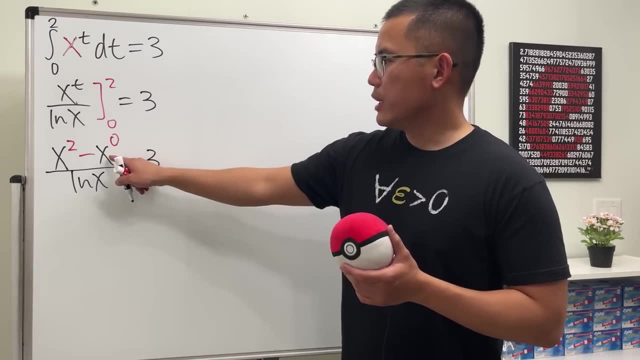 power, And both of them have the ln x. so I'm just going to put that down right here like this: and this is equal to 3.. Okay, and then perhaps we can write this down: x to the 0's power as 1,. 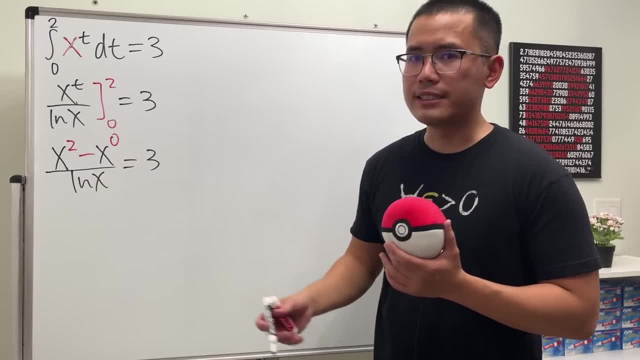 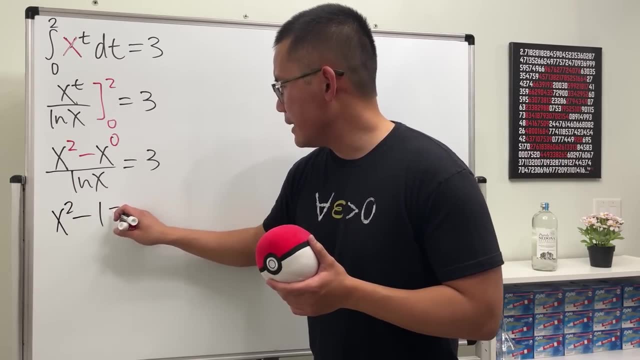 and maybe we can multiply the ln x on both, Because usually we don't like to see fractions in the equation. So we are getting x squared minus 1 being equal to 3 ln x. Now how in the world do we solve this kind of equations? 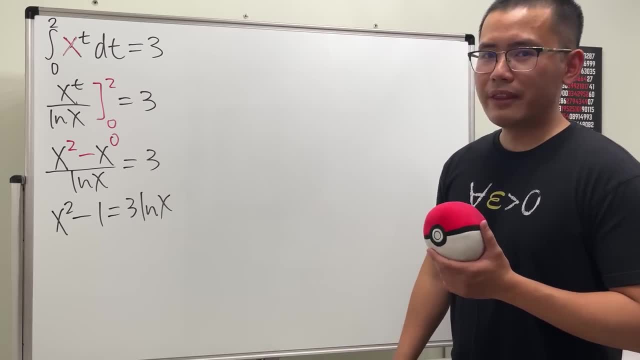 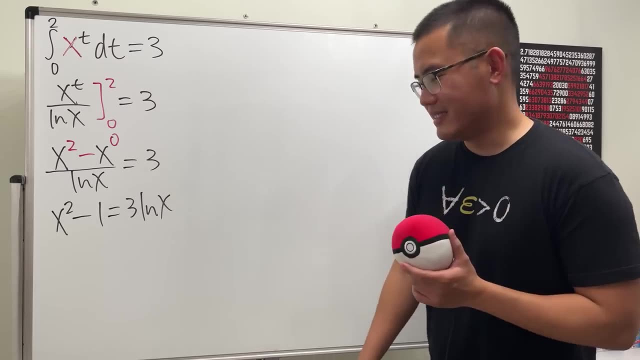 Right, Newton's method. No, no, no, no, no, no. I know it works, but let's try the Lambert method. What's the Lambert? What's the Lambert-W function? And here's the idea like: how do we know to use the Lambert-W? 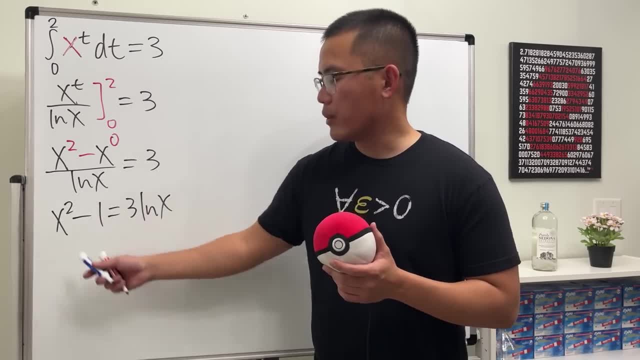 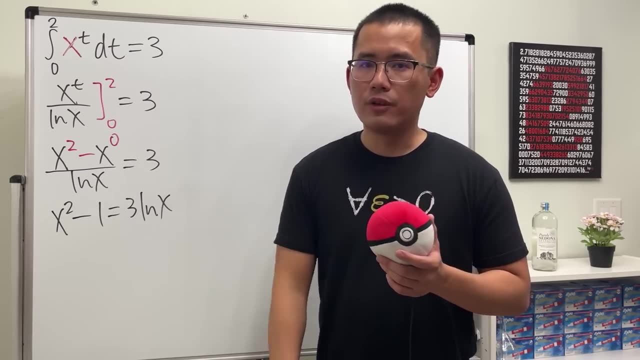 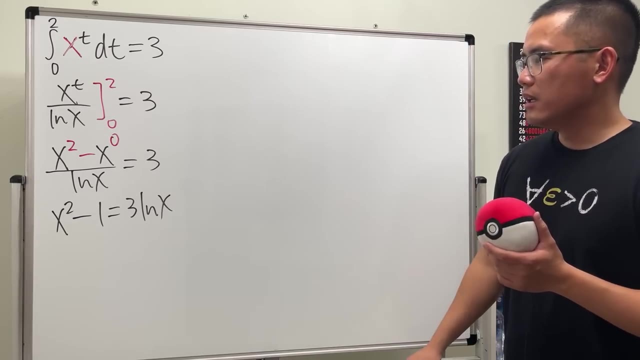 function. When we have a power function, x to some power and then natural log or exponential e to the whatever- sometimes the Lambert-W function might be able to help us out. So just keep that in mind. I'm not saying all the time, but just keep that in mind And I would like to write down. 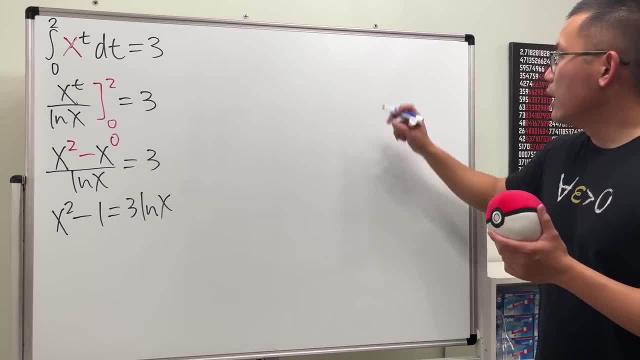 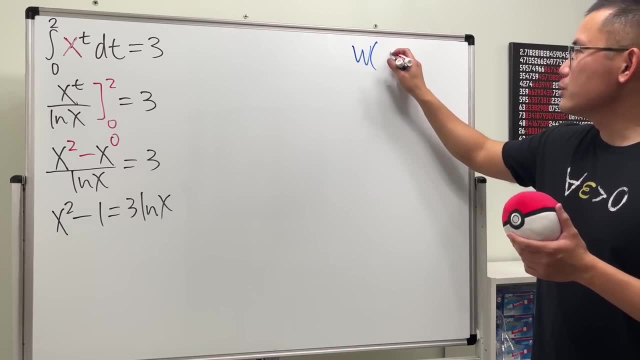 the most important note for you guys when we use the Lambert-W function. I'll put it down right here And I know you guys like me to draw the fish, so I will give you guys the fish. Suppose we have a fish in the front, This is not alpha, This is a fish. It's a happy face Times e like the special. 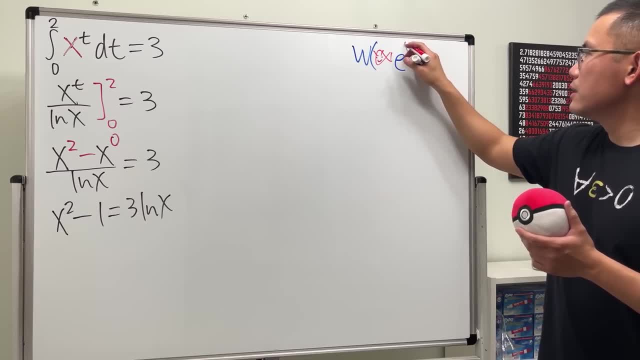 constant e raised to the same fish. All right, If this and that are the same, and once we apply the Lambert-W function, guess what? We will just get the fish back. And this, right here, is the most important part of using the Lambert-W function. So let's just put the fish back. And this, right here, is the most important part of using the Lambert-W function. 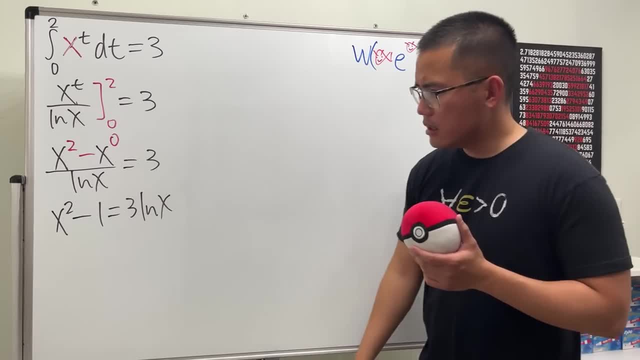 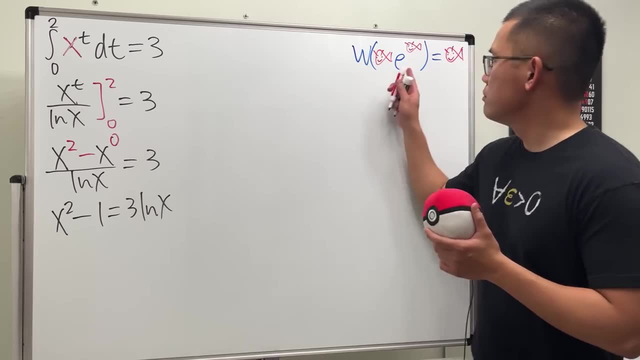 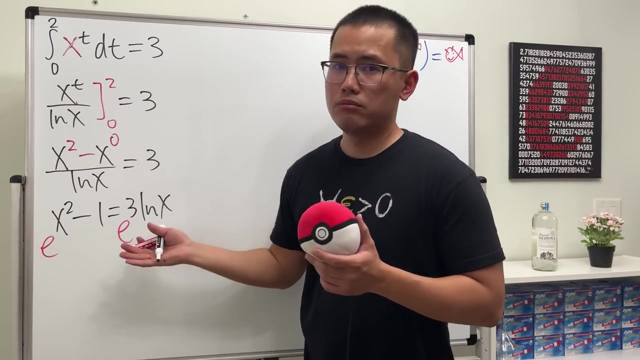 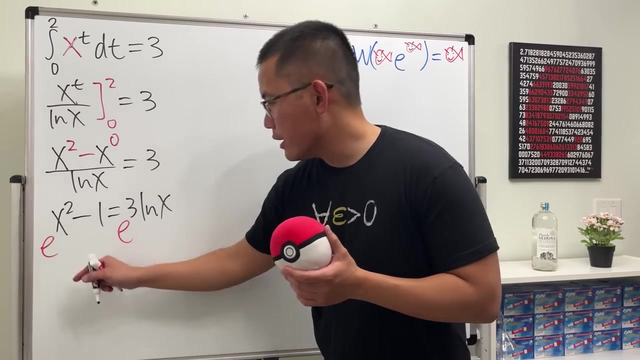 w function. so, with that being said, we kind of want to introduce the e to help us out a little bit, don't you think so? all right, so what we can do is let's just do e to this power and e to that power. all right, cool. on the 11th side, we have x squared minus 1 in the power. let's break them apart, so we 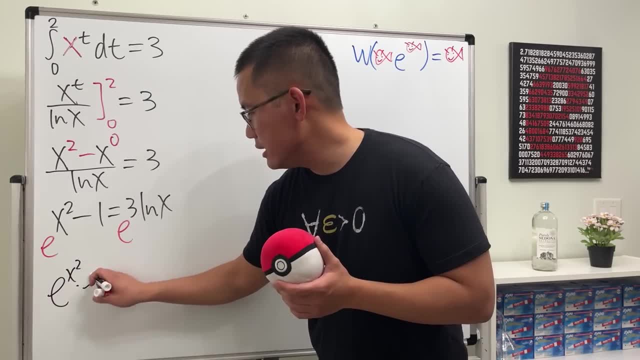 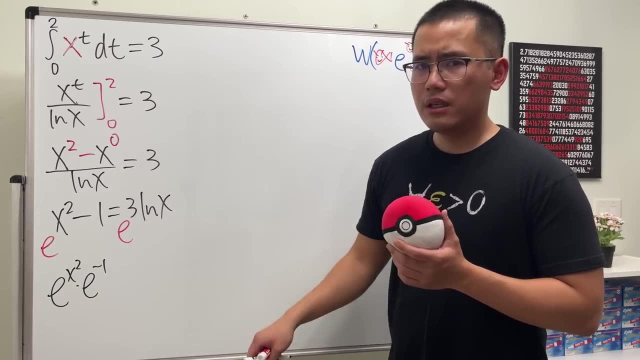 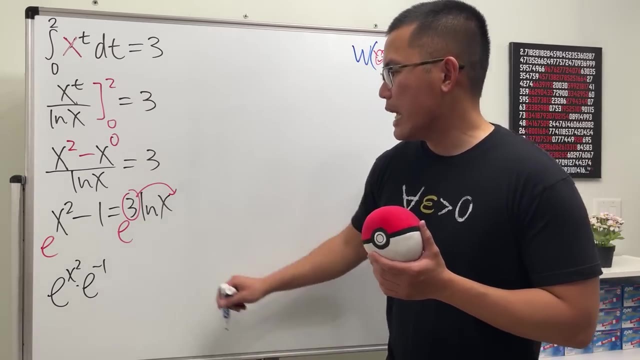 will get e to the x square times e to the negative 1. that's the jet. and then for the right hand side we have the e and ln. but we cannot cancel it out yet. we will have to first put the 3 back here for the to become the power and then cancel the e and then ln. so the right hand side gives us x to the. 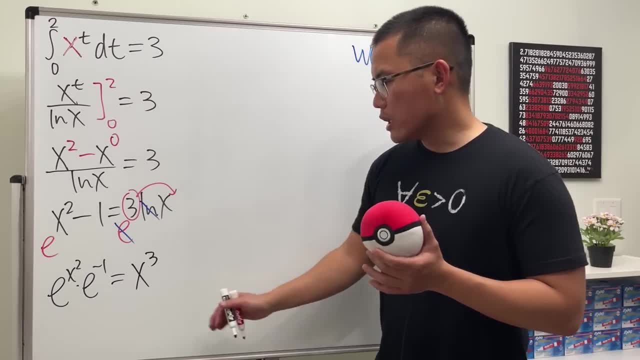 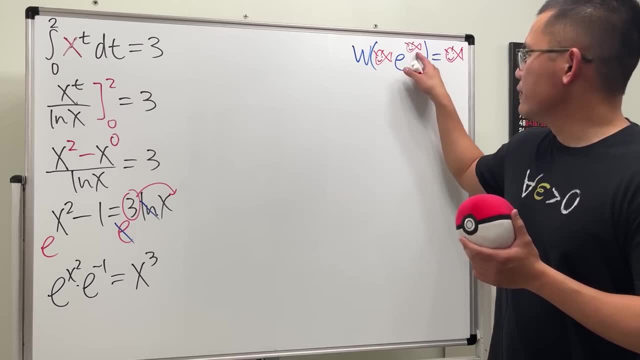 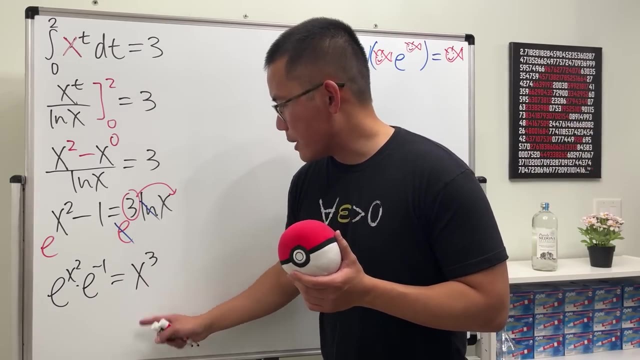 third power, all right. so now we are working with power and also exponential, all right. and you see, we kind of want to have the fish and fish on the same side. i want to have the function part being on the same side. so let me divide the x to the third power on both sides and let's kick. 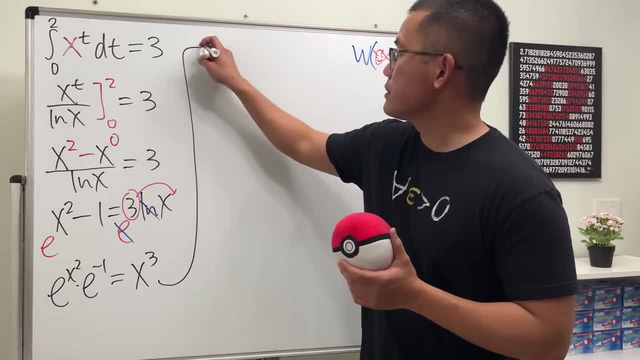 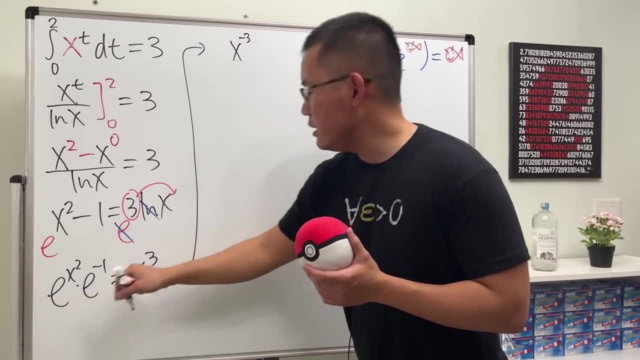 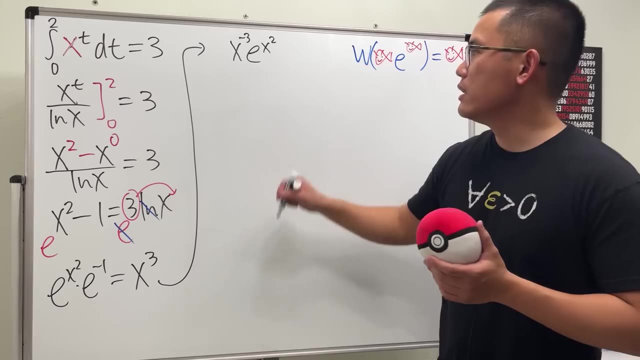 the number to the other side, and this is what we are going to get. divide this to the other side, we will get x to the negative 3 power and then we have e to the x squared power and then we divide this on both sides 1 over e to the negative 1. 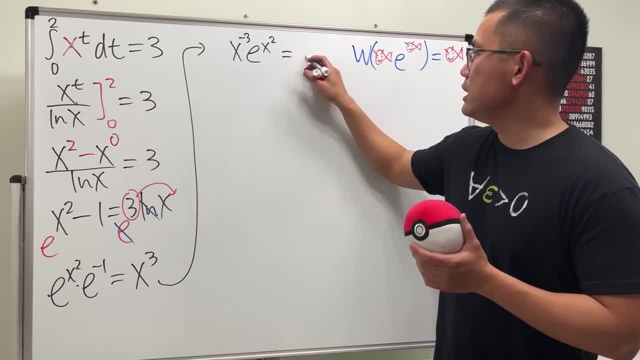 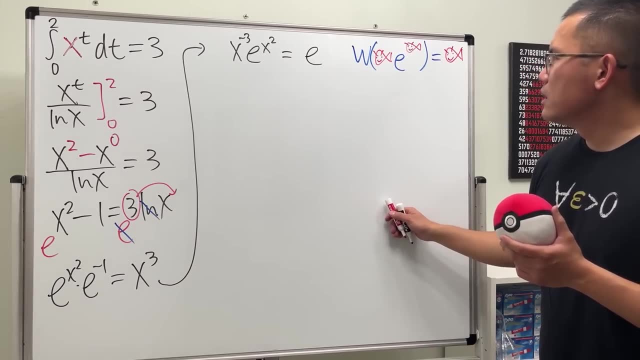 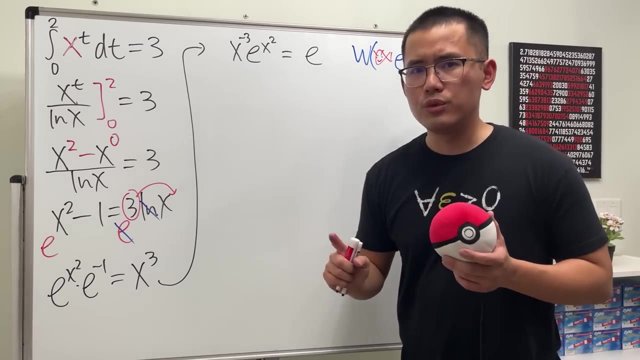 and then we have e to the first power, so i'm just going to write this down as just e. cool, i think we are making a good progress. notice: here: we have x squared, but this is x to the negative 3. we don't want a negative 3, we want to have this right here being 2 as well. how can we make that happen, though? 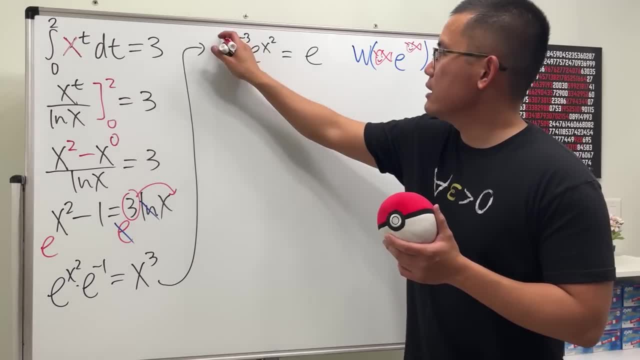 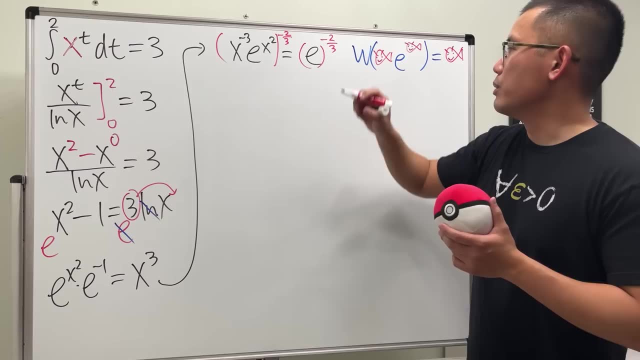 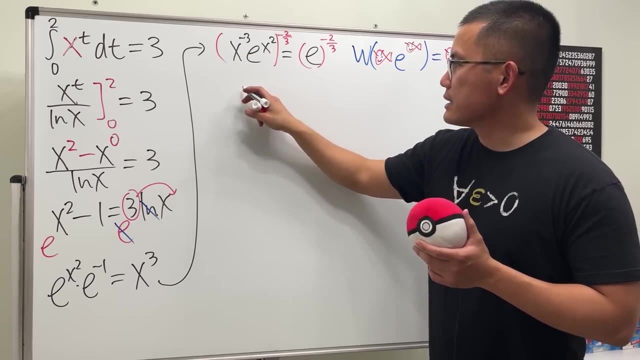 well, this is the power. so what we can do is just go ahead, raise both sides to the negative 2 over 3 power, and of course we do it to both sides because this way we can distribute the power and inside just a multiplication, so we will just get x negative 3 times that. 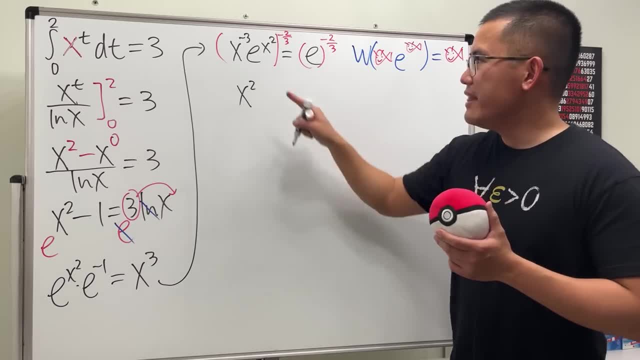 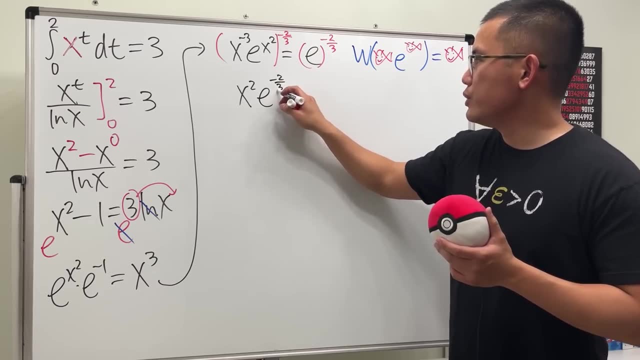 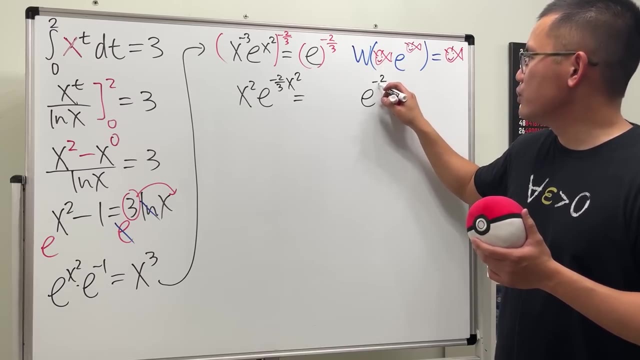 we get positive 2.. very nice, huh. and then when we distribute the power, we do x squared times that, so we get e to the negative 2 over 3 x squared power, and this right here gives us e to the negative 2 over 3.. i know it looks pretty crazy now. 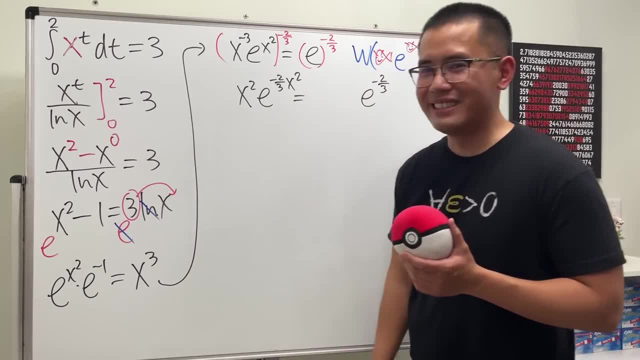 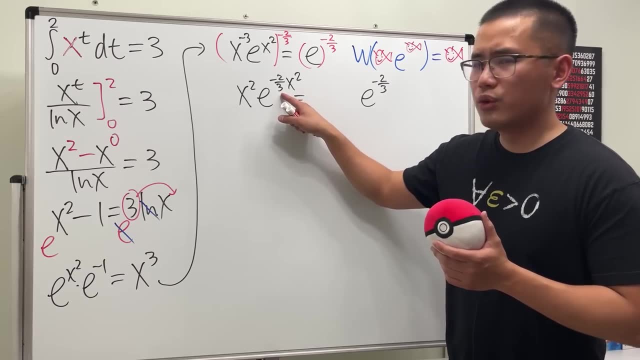 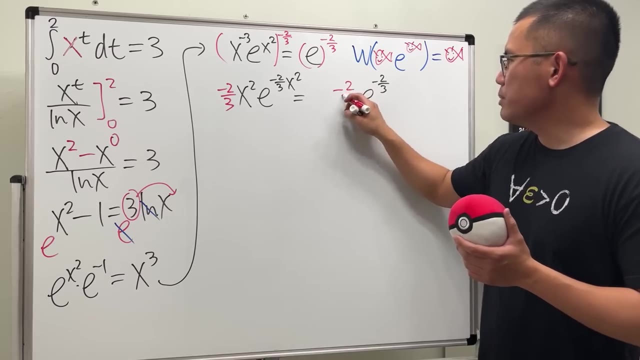 yeah, you have. it has been crazy, like maybe right here already. all right, that's pretty good, but now we need to have the negative 2 over 3. we're almost there, so what can we do? yeah, just multiply that on both sides. we need a negative 2 over 3. let's multiply negative 2 over. 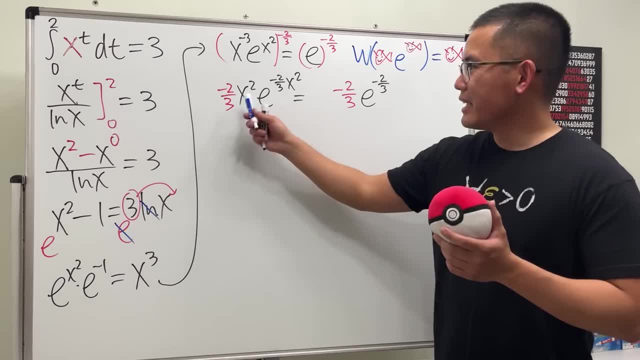 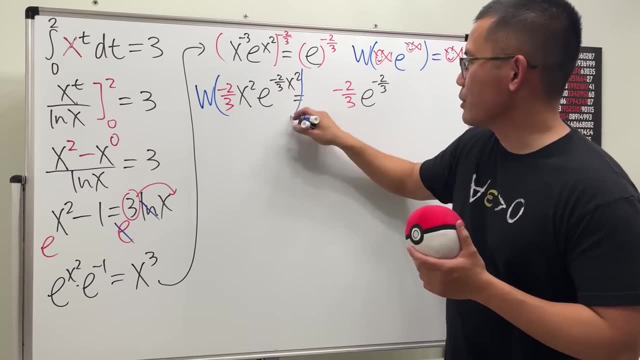 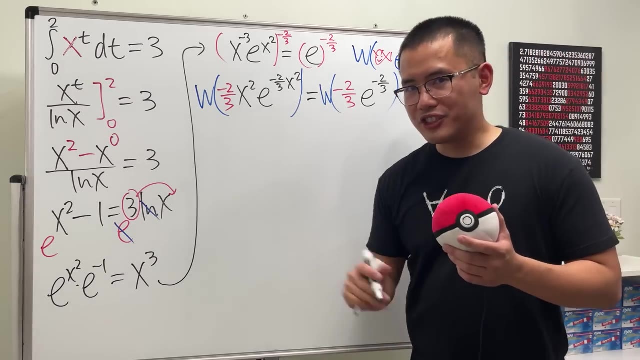 3 on both sides. and then, ladies and gentlemen, here we have the fish and here we have the same exact. therefore, we can just go ahead and take the happy limber w function on both sides like this, cool, and now check this out on the left hand side. this and that are the same, so just like. 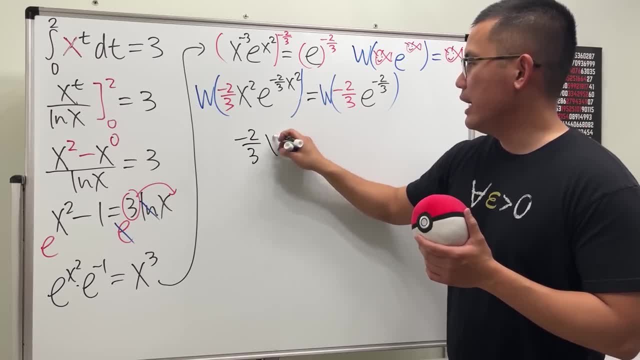 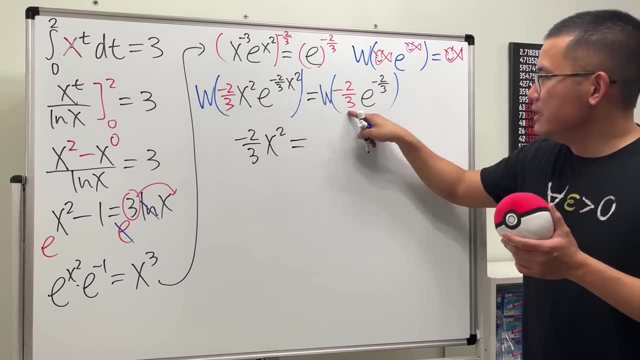 that we know we will just get negative 2 over 3 x squared, done on the right hand side. you might notice this is very interesting because this and that are the same. so by this again, hey, we should just get negative two over three right here as well, right? 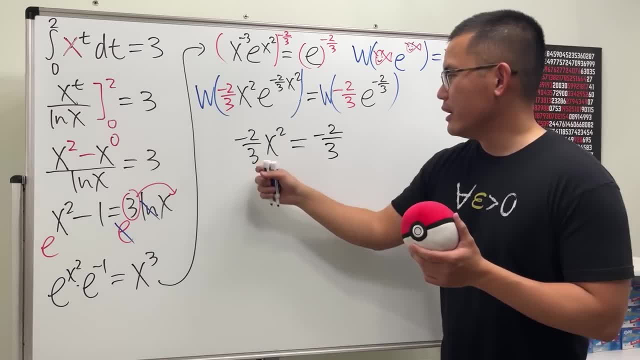 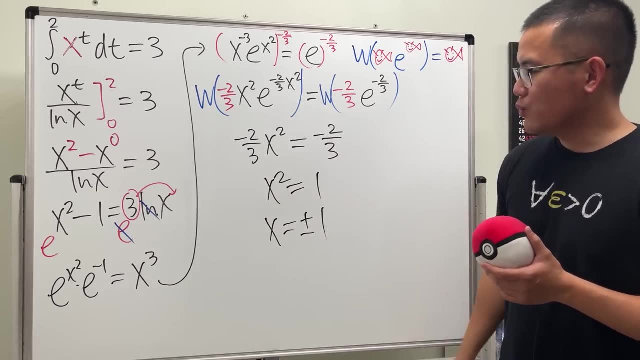 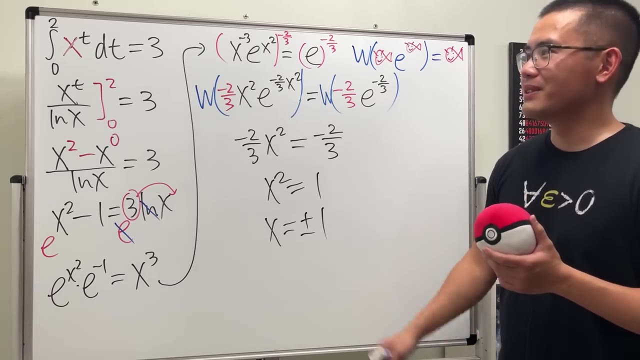 and guess what? let's continue. divide this on both sides. we get x squared is equal to one and do the usual business. we are saying axis should be plus or minus one done? no, this is not correct. this is not correct. why, if we put one back to the original equation, 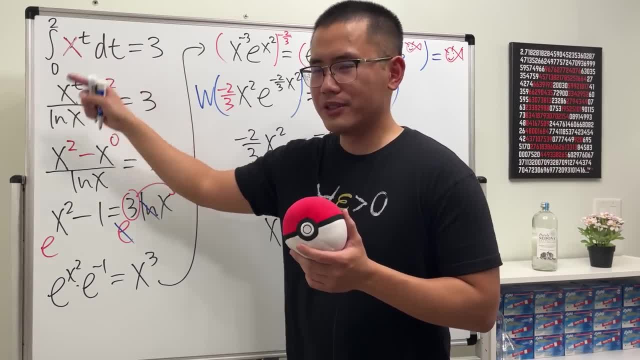 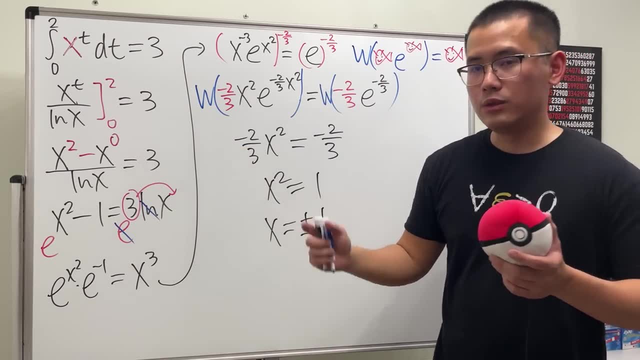 this is an equation, okay, so we're gonna do this again. so again, this is the original equation. so by this again, hey, we should just get negative two over three right here as well. right equation, which is the one in here, one to the t's power is just always equal to one. right in the 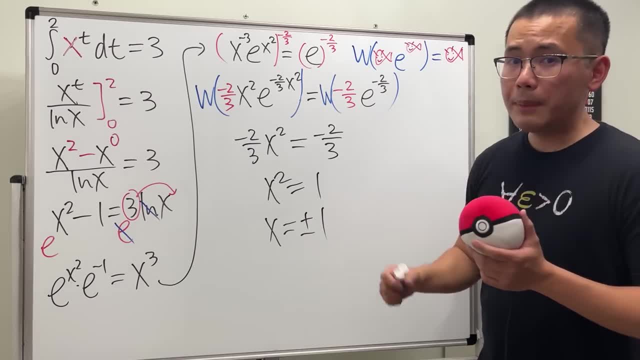 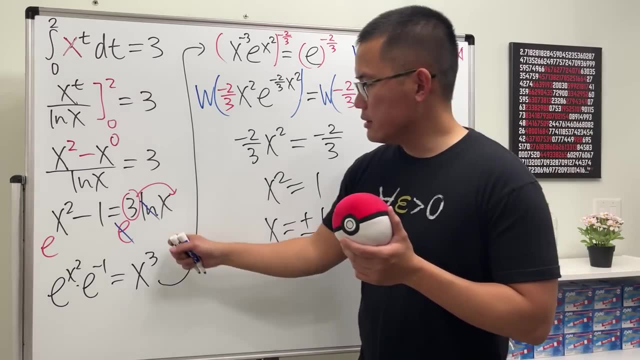 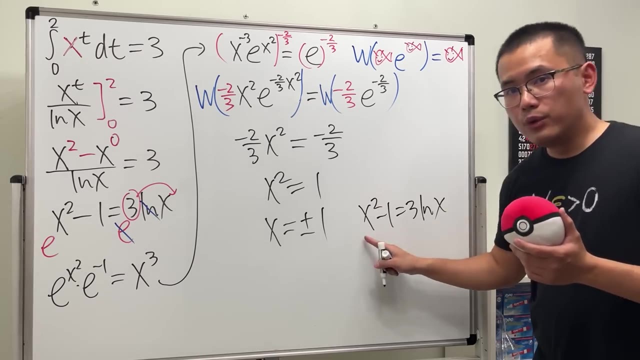 real world. so this right here does not work. and now you might be wondering: how did this process give us one for the answer though? well, i'll tell you: it's because it's right here. when we had x, squared minus one is equal to three times l and x. if you look at just this equation. 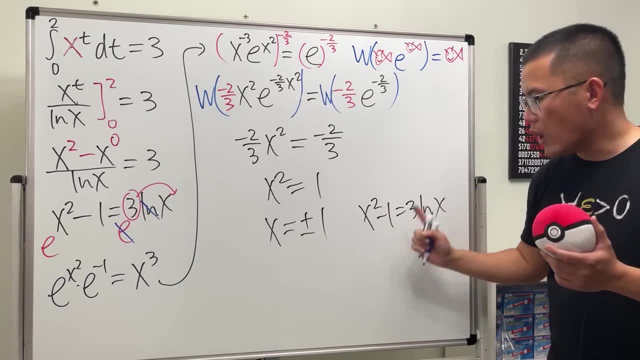 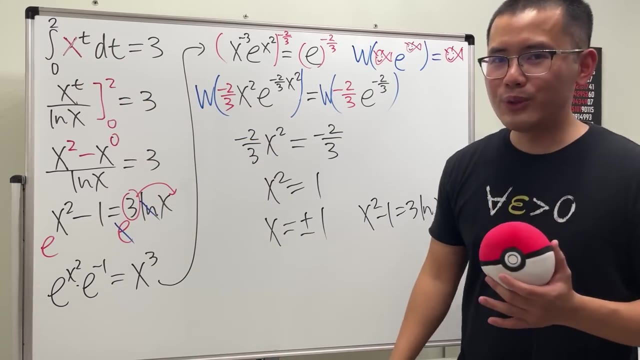 right, nothing else. then let me tell you one is indeed a legitimate answer to this equation, because you will get zero on the left hand side and also zero on the right hand side, but you always, always have to refer back to the original equation to see what we are trying to do, and then 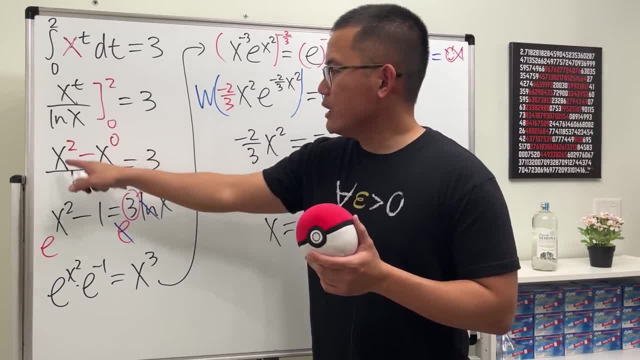 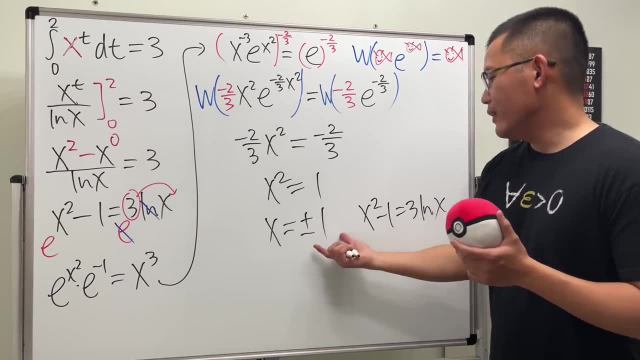 get rid of the one. in fact one wouldn't apply once we get to here, because we get l and one which is zero on the bottom. that doesn't work either. and then negative one is just our right hand side, and we will get electric and we will get x squared, which is zero on the bottom. 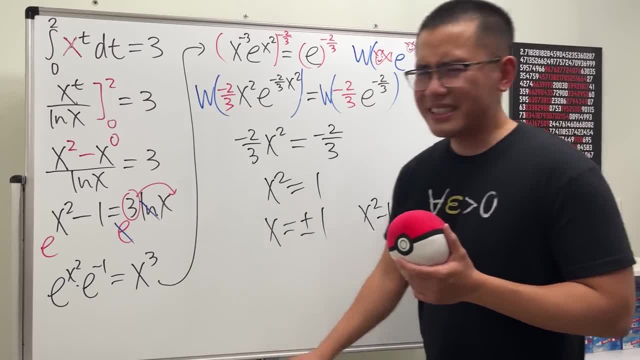 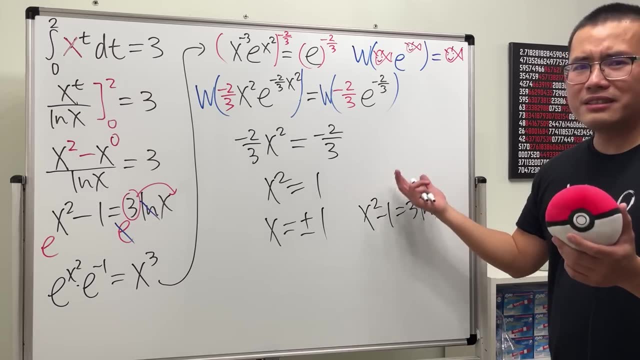 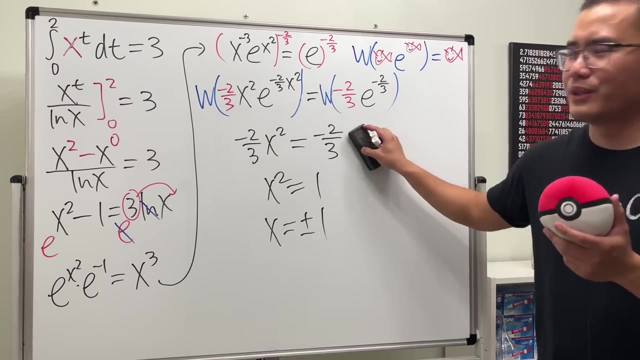 outrageous, so let's not even talk about that. so why exactly did this go wrong, though? did the number w function fail? because where's my answer? right? so hopefully by now you guys should see why this is hard, and of course I have the answer for you guys, don't worry. 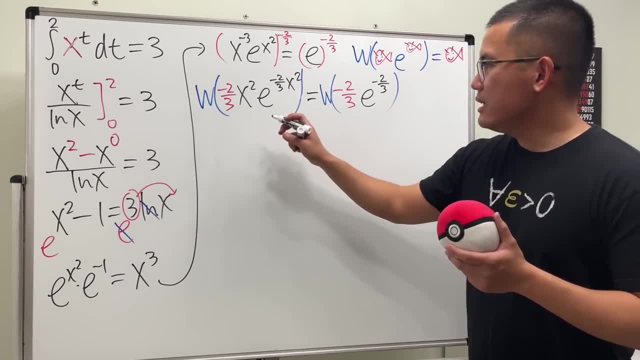 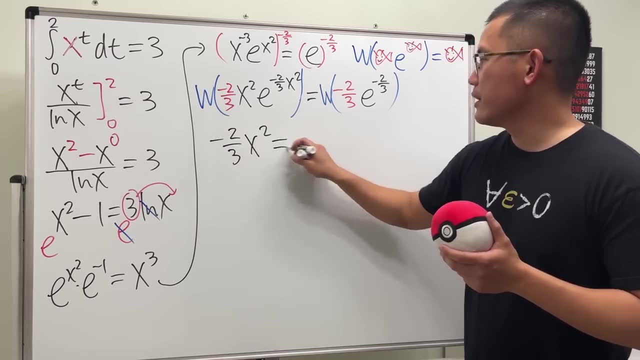 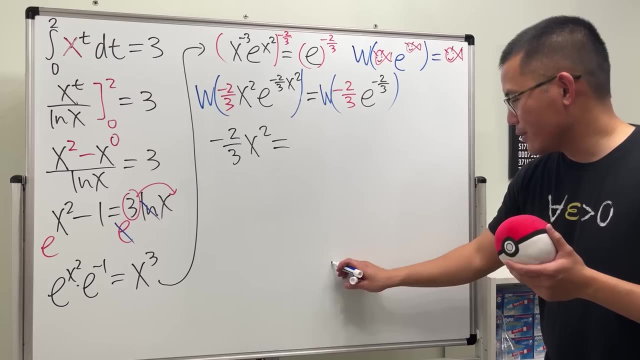 I would like to tell you guys this, on the left hand side, it's okay, I will just write it as negative: 2 over 3 x squared, that's okay. on the right hand side, I would like to tell you guys, with some more notes on the side right here: 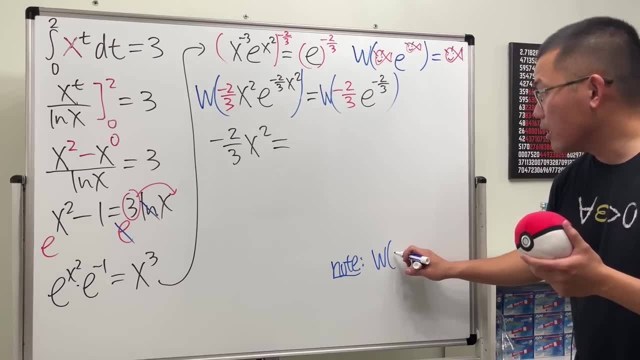 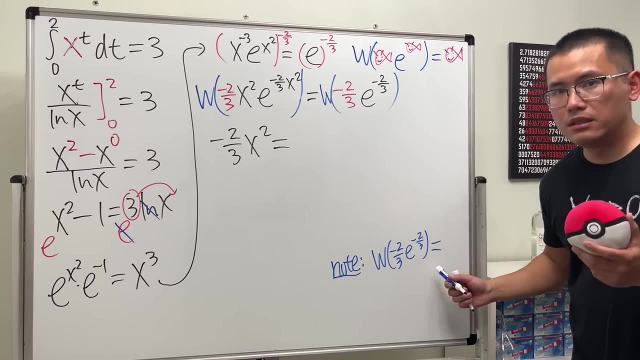 earlier. when we just look at the number w function of negative 2 over 3 e to the negative 2 over 3 power. this right here will indeed give you negative 2 over 3, because this and now are the same good, but this is the so-called principal value or the principal branch. it's kind of like saying the 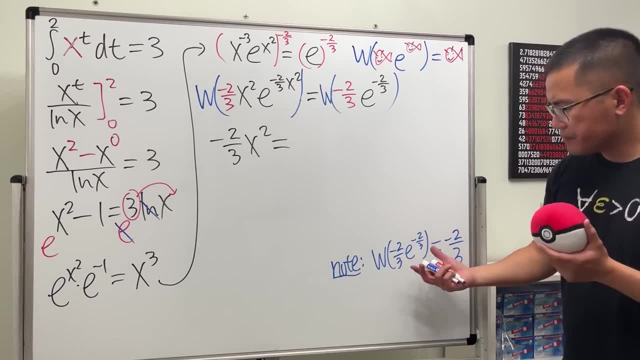 first answer and to make the principal branch clear. usually we say w with a subscript zero here. all right, and that's why they use a warfarin alpha as well, but unfortunately the principal value does not help us to solve this equation. so what do we do then? just go to another branch? 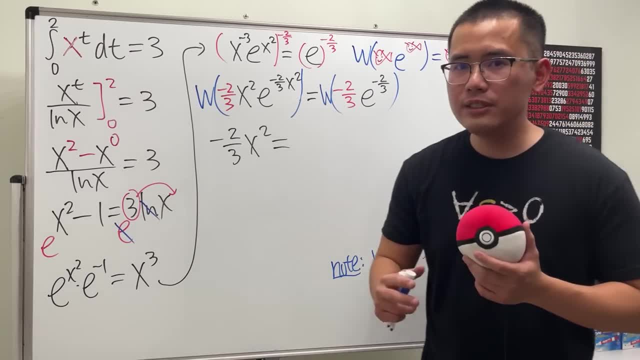 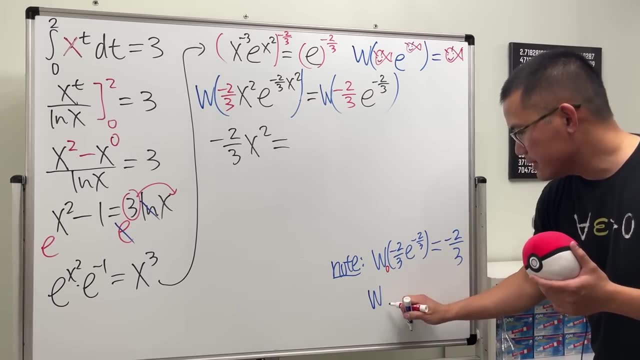 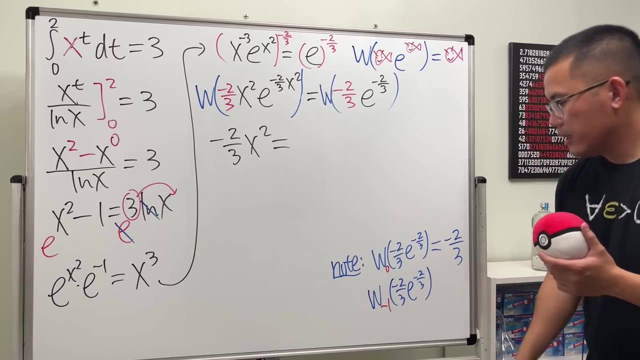 another branch and let me tell you, we will actually still end up with another real solution once we get to another branch. so what's the other branch, I will tell you, is the negative 1 branch and we get negative 2 over 3 e to the negative 2 over 3. you can use w alpha for this and I have the answer written down over. 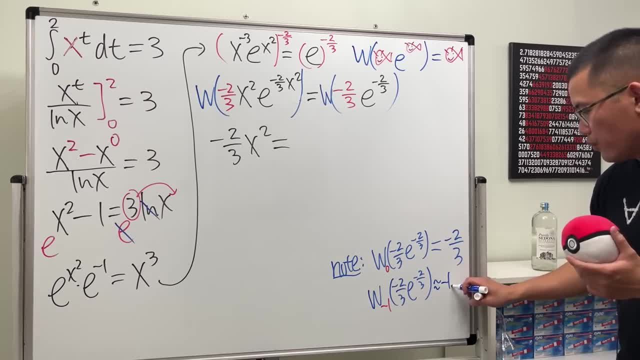 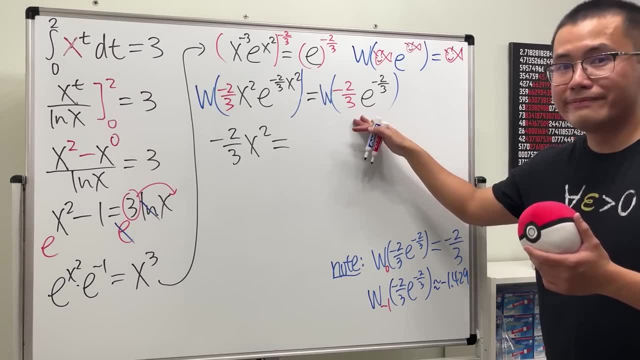 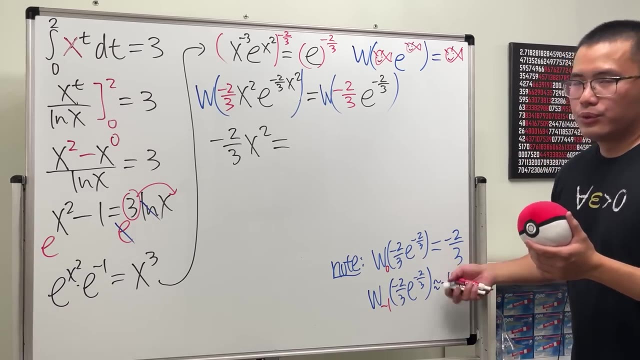 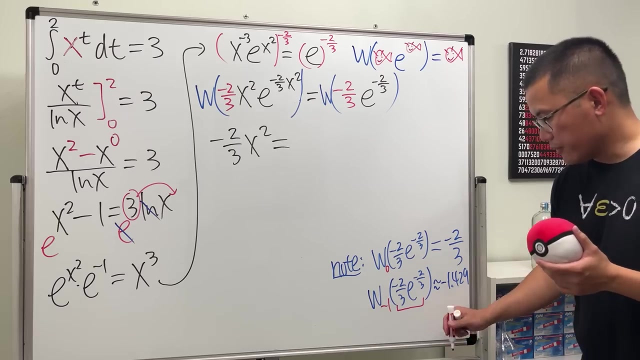 there already. this right here is approximately negative 1.429. so this is the answer that we are going to use right here. all right, and now you may be wondering why? why does this give you two answers. let me tell you: pay close attention to the input, this number, if it's in between of- well, 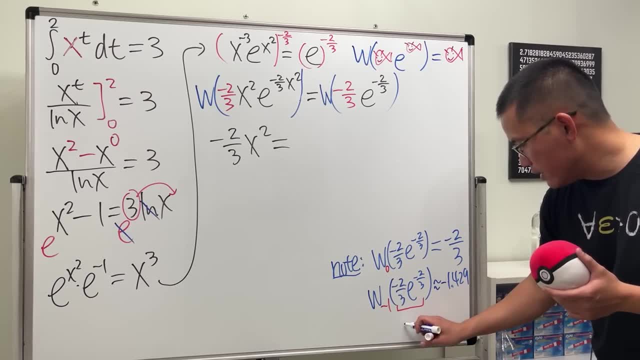 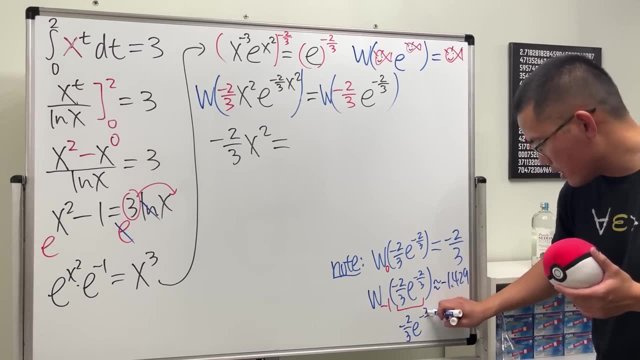 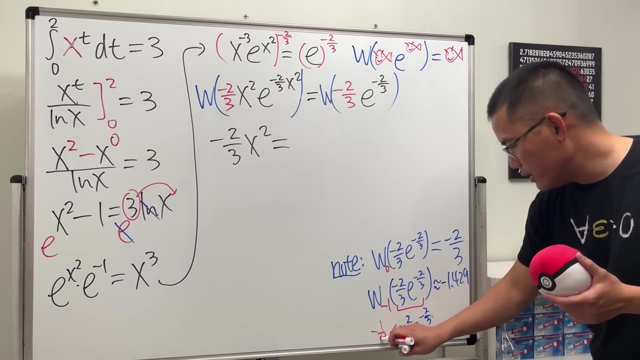 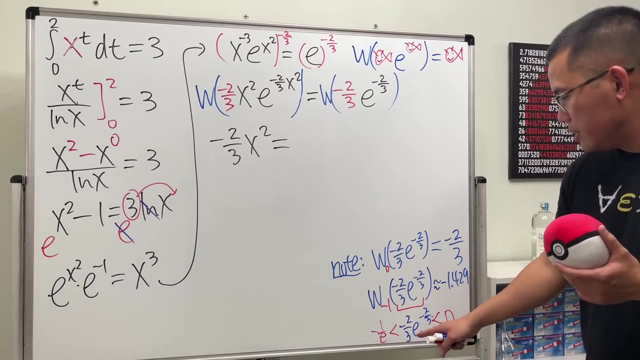 let me write it down: this number which is negative 2 over 3, e to the negative 2 over 3. if this is in between of negative 1 over e and 0, then we are going to have two answers. right, we are going to have two answers and let me just tell you guys that this right here, 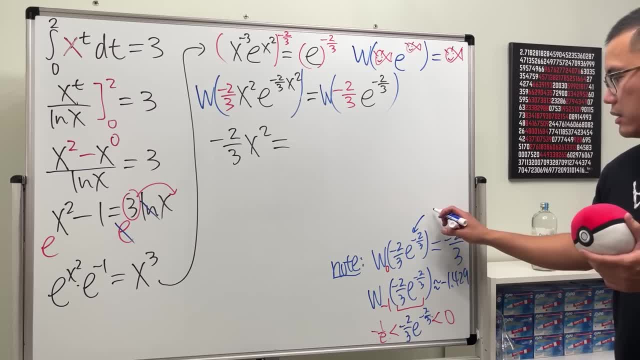 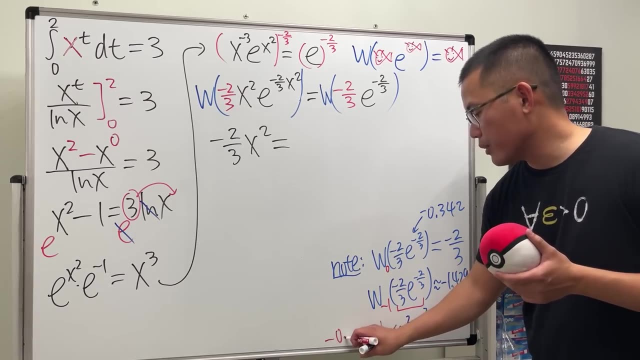 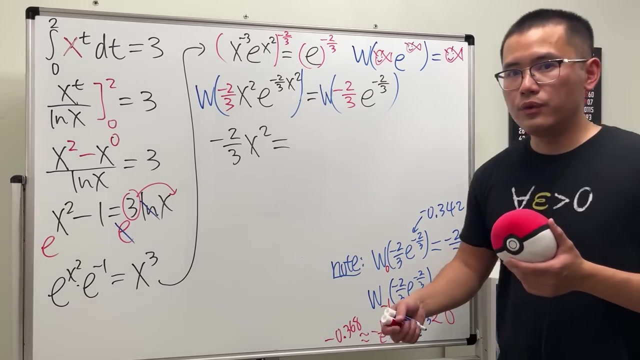 and this number right here is approximately zero point three, four, two, just kidding, it's negative. and this number right here, negative 1 over e, is negative 0.368. all right, so that's why, you see, this is indeed between this and that. that's why it will give you two answers. when we use the number w function and you might. 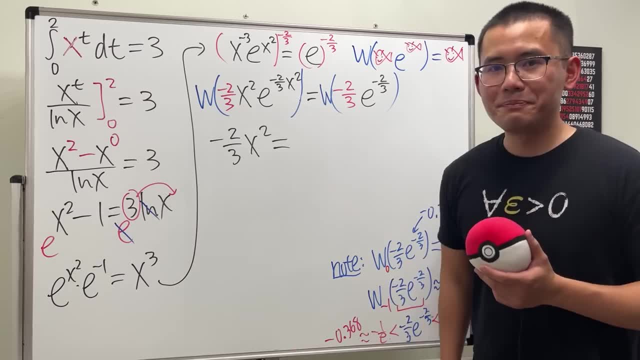 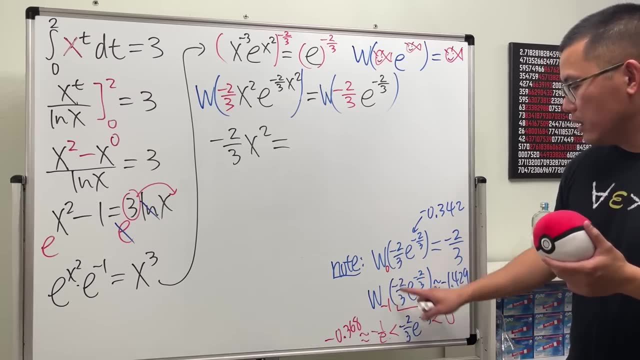 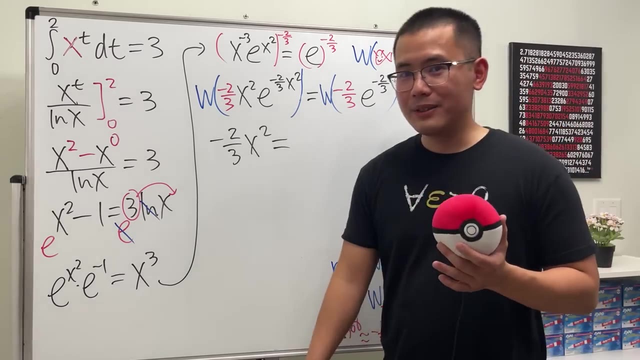 be wondering: are there any more answers? yes, if you go to the other branches, such as the negative 2 branch or such as the first branch, you end up with a lot more answers and in fact, they are all common, complex answers. so yeah, it's really crazy, huh. i would like to keep the answer in the exact form.